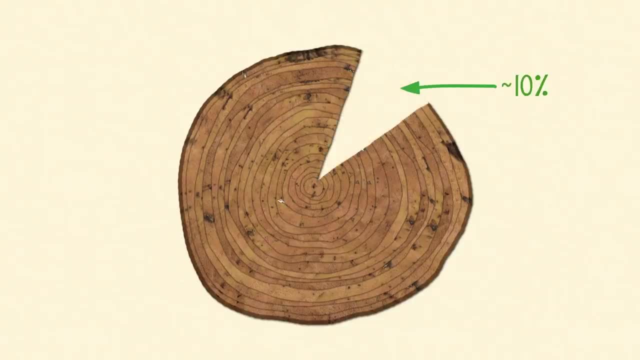 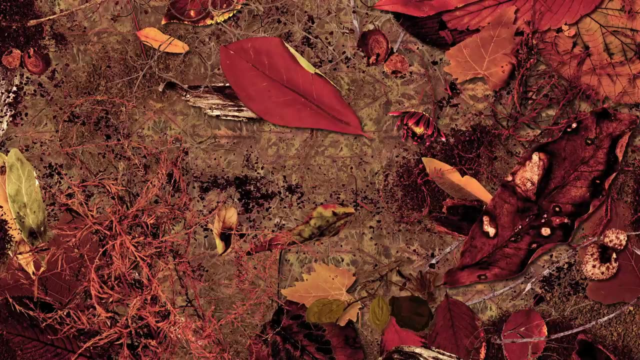 But in real-life terrestrial ecosystems, less than 10% of plant matter is eaten while it's still alive. What about the other 90?? Well, just look at the ground. It's on an autumn day. Living plants shed dead body parts. 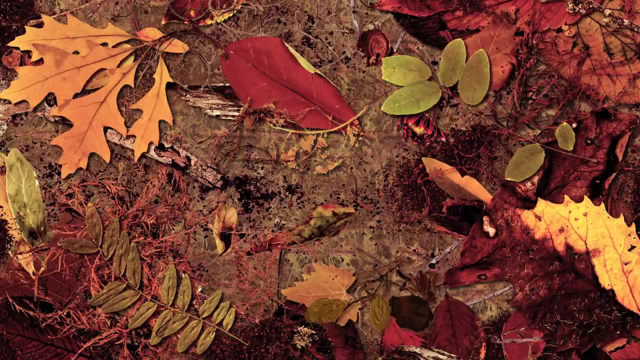 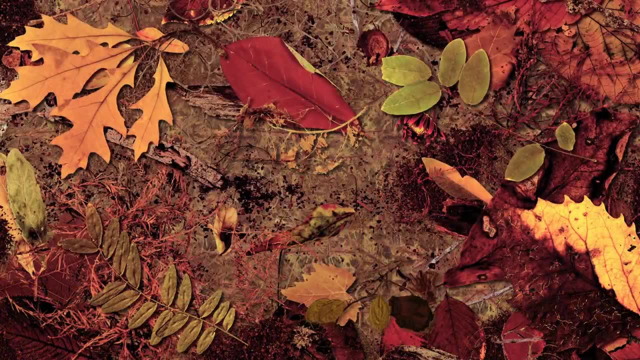 fallen leaves, broken branches and even underground roots. Many plants are lucky enough to go their whole lives without being eaten, eventually dying and leaving remains All of these uneaten, undigested and dead plant parts that 90% of terrestrial plant matter. 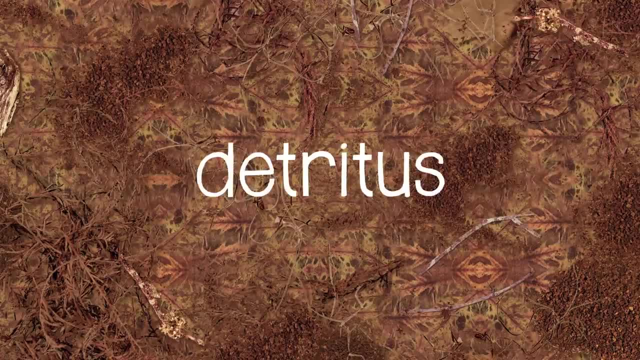 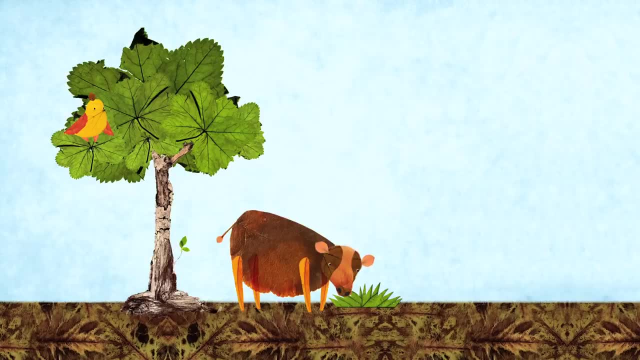 that becomes detritus, the base of what we call the brown food chain, which looks more like this: What happens to plants also happens to all other organisms up the food chain. Some are eaten alive, but most are eaten only when they're dead and rotting. 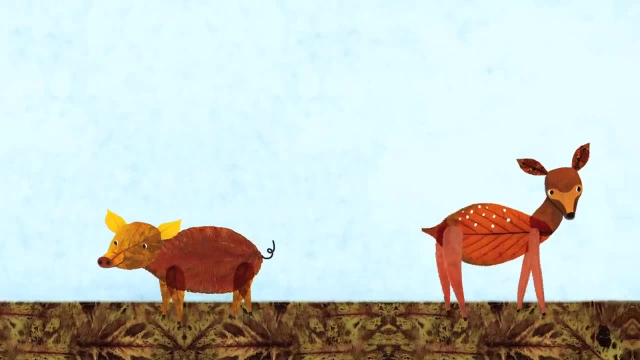 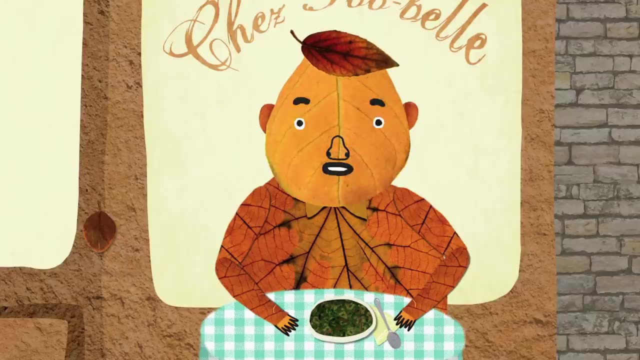 And all along this food chain, living things shed organic matter and expel digestive waste before dying and leaving their remains to decay. All that death sounds grim, right, But it's not All. detritus is ultimately consumed by microbes and other scavengers. 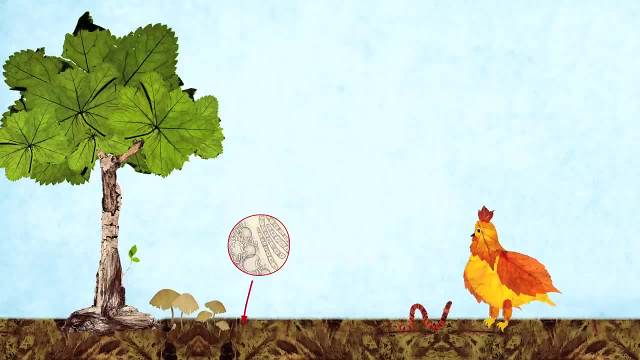 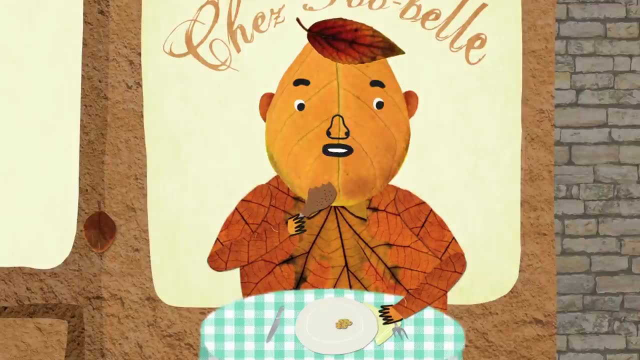 so it actually forms the base of the brown food chain that supports many other organisms, including us. Scientists are learning that this detritus is an unexpectedly huge energy source, fueling most natural ecosystems, But the interactions within an ecosystem are even more complex than that. 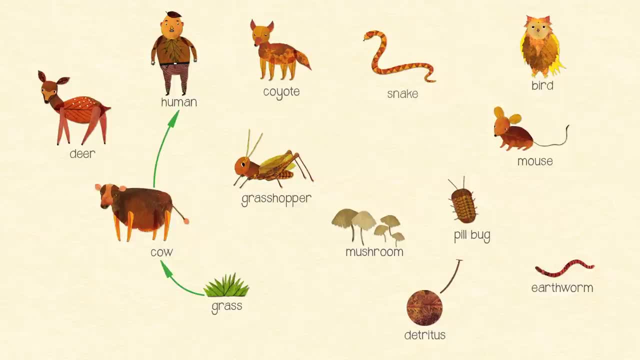 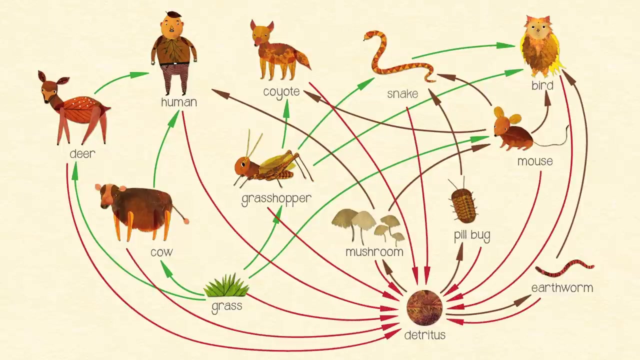 What a food chain really represents is a single pathway of energy flow And within any ecosystem, many of these flows are linked together to form a rich network of interactions, or food web, with dead matter supporting that network at every step. The resulting food web is so connected. 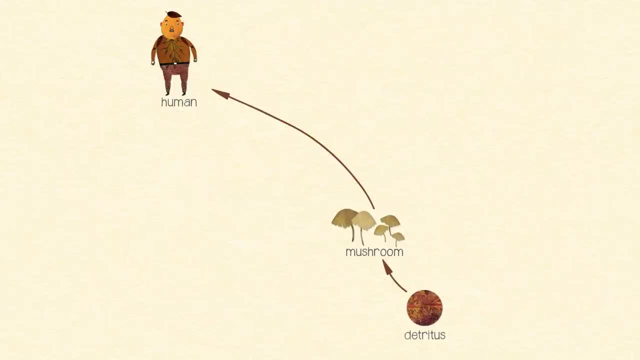 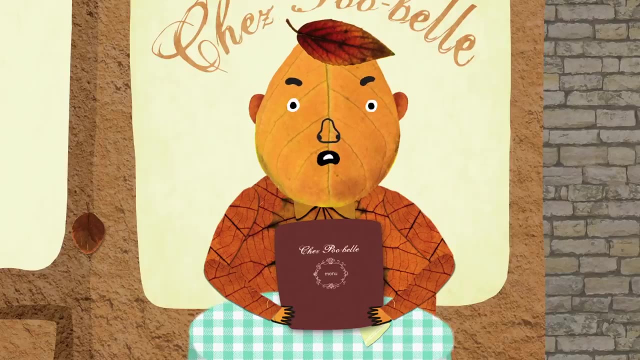 that almost every species is no more than two degrees from detritus. even us humans. You probably don't eat rotting things- poop or pond scum- directly, but your food sources probably do. Many animals we eat either feed directly on detritus themselves. 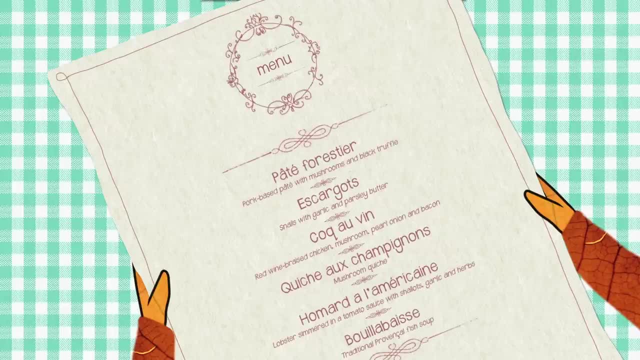 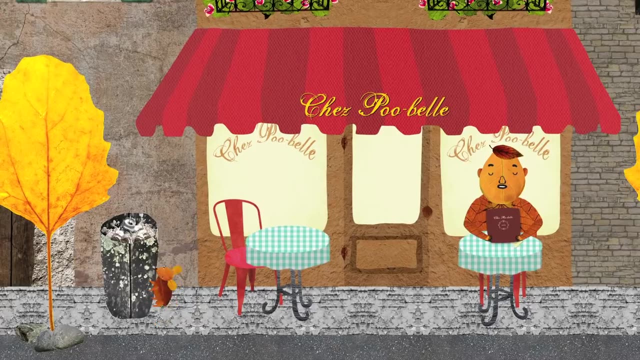 like pork, poultry, mushrooms, shellfish or catfish and other bottom feeders, or they're fed animal byproducts. So if you're thinking that nature is full of waste, you're right. But one organism's garbage is another's gold. 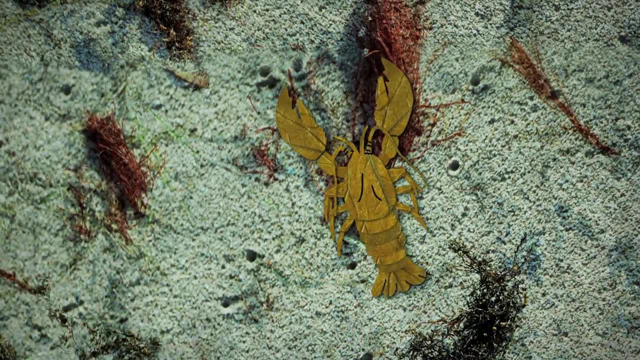 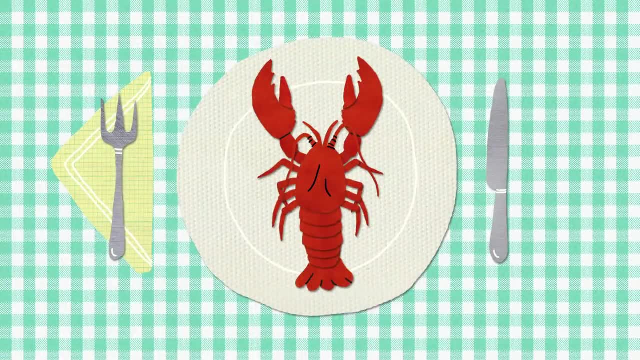 And all that rotting dead stuff ultimately provides the energy that nourishes us and most of life on Earth as it passes through the food web. Now that's some food for thought.